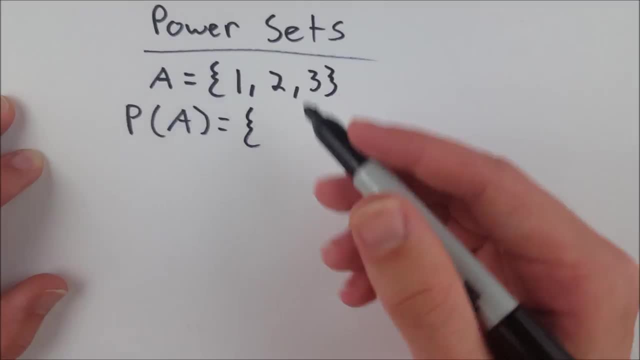 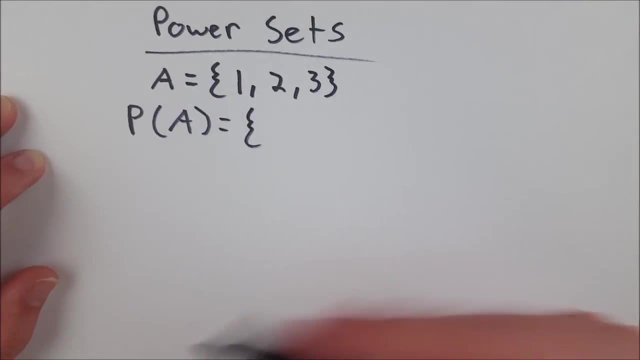 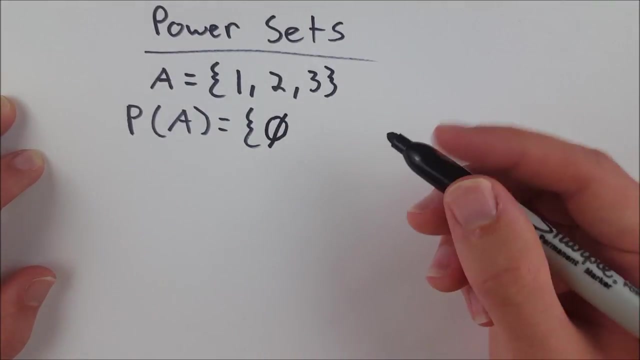 is equal to the set that contains every subset of A. So all you have to do is open up a set, put in this set every subset of A and that's your power set. So let's do this example For starters. we have the empty set, because the empty set is a subset of every set. 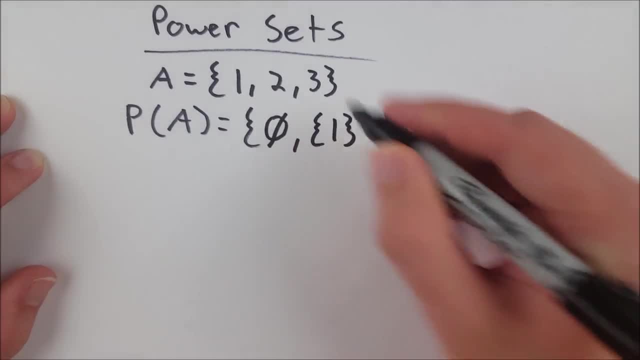 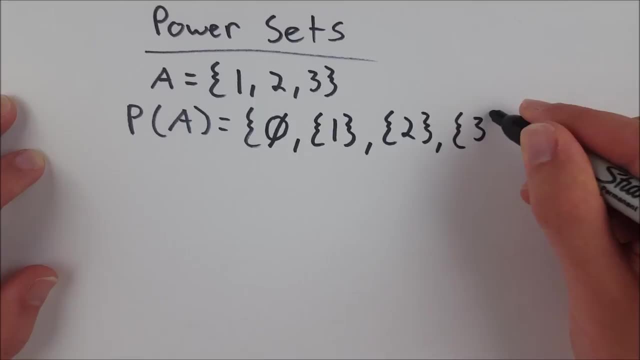 Then we have the set containing 1.. This set's a subset of A. We have the set containing 2.. That's a subset, Remembering that a subset of one set is any set whose elements are all present in A. So let's continue. We have the set containing 1, the set containing 2, the set containing 3, the set containing 1 and 2.. 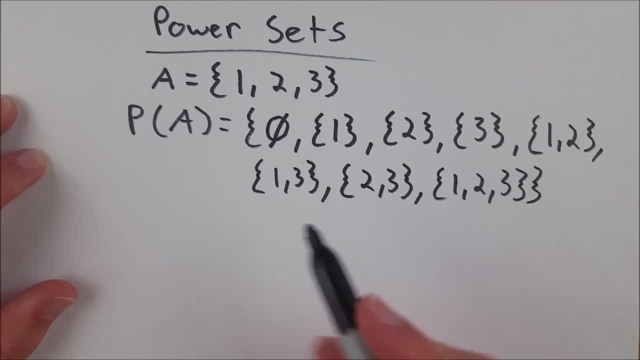 And I'll just write the rest of these out and we'll skip to that And that is our power set. I'm sorry that it spans two lines. It makes it a little tougher to look at, But that's the power set. So in this set, 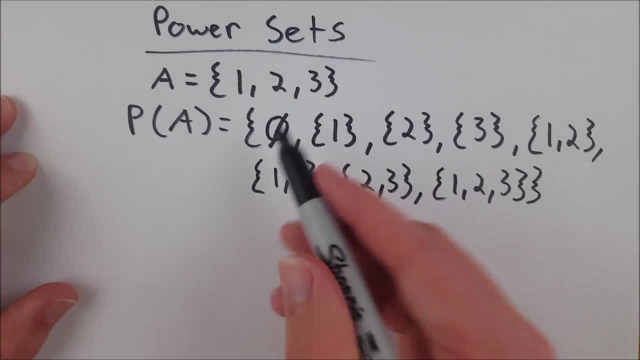 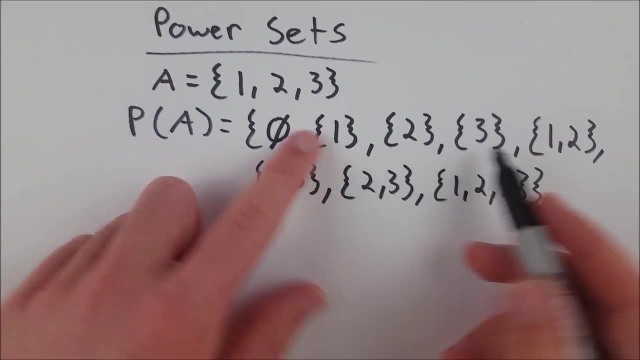 The power set of A is every subset of A. We have the empty set, which is a subset, and then we have all the sets that contain elements present in A: 1, 2,, 3, 1, 2.. 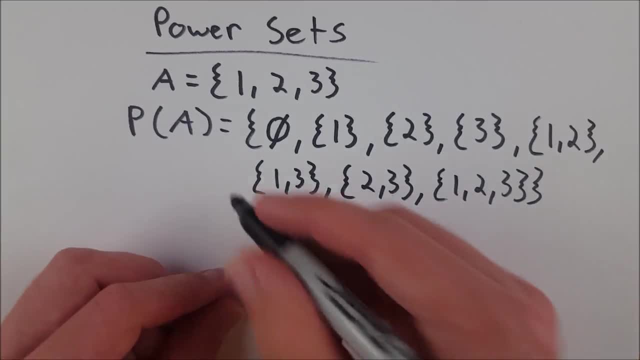 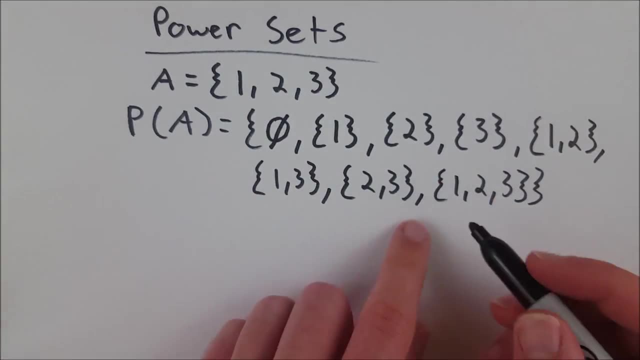 Again, rule of a subset is that if A, let's say if a little a- is an element of this set, then it must also be an element of this set. That's what makes it a subset, which is why the set itself we see, A, is in here as well. 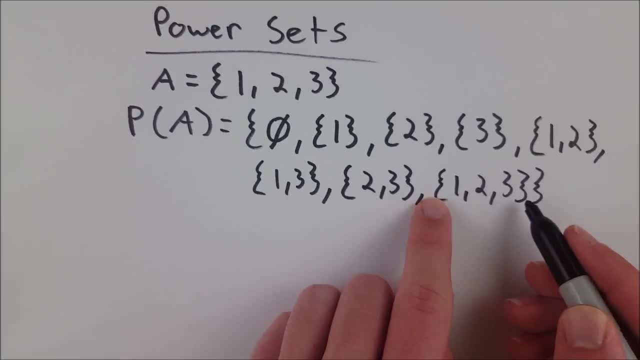 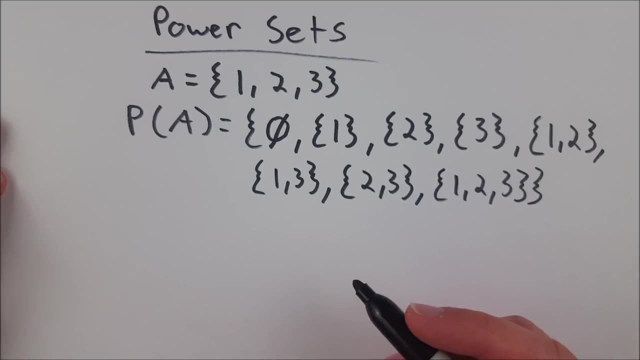 that set is also a subset of A, because every element in this set is also in this set And we can sort of check ourselves when we're writing power sets with a simple rule: The amount of subsets that any given set has is 2 to the power of n. 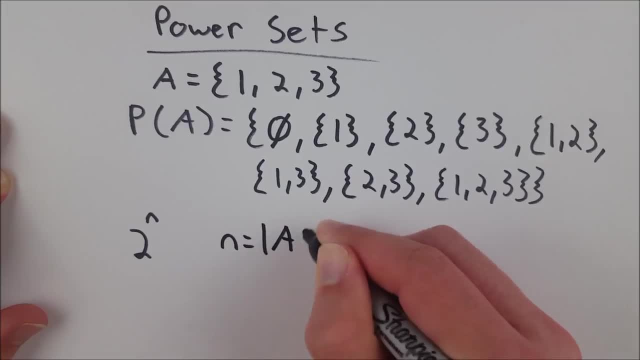 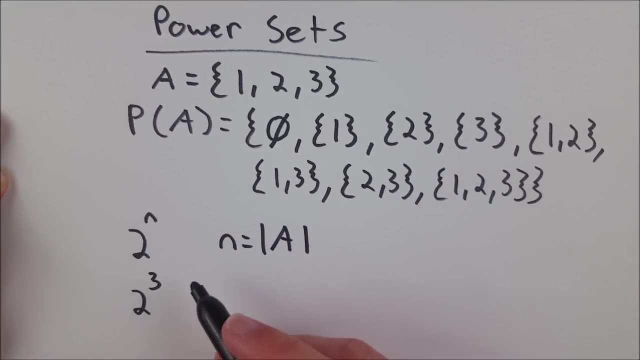 where n is the cardinality of the set. In this case that will be 2 to the third, because A has a cardinality of 3.. So there should be Well, that means that there's 8 subsets of A. 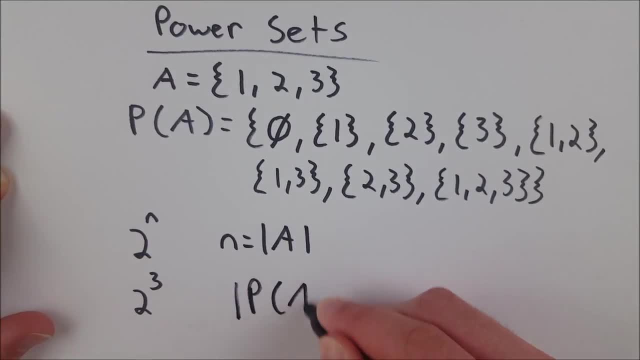 Therefore the cardinality of our power set should also have 3 subsets, be 8, because again, the power set is the set containing all subsets. you see here: 1, 2, 3, 4, 5, 6, 7, 8. that checks out a. okay, the cardinality of our power set is a as: